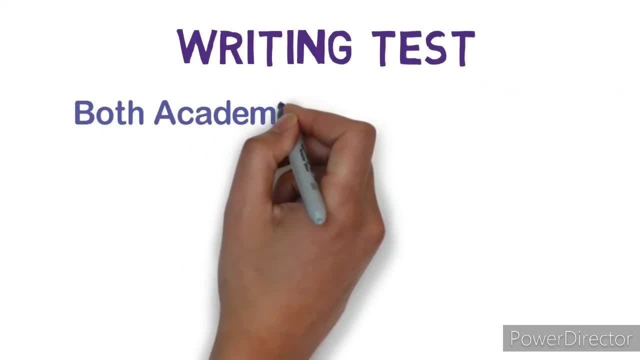 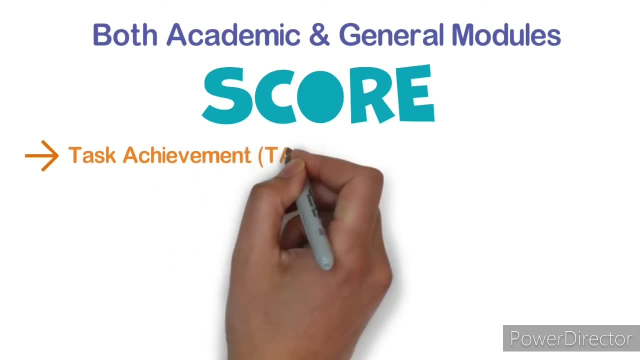 In the writing test for both academic and general modules. your scores depend on 4 different factors. First one is the task achievement, or TA. It includes that you are making enough paragraphs and you have written enough words in your writing test. The second one is coherence and cohesion. 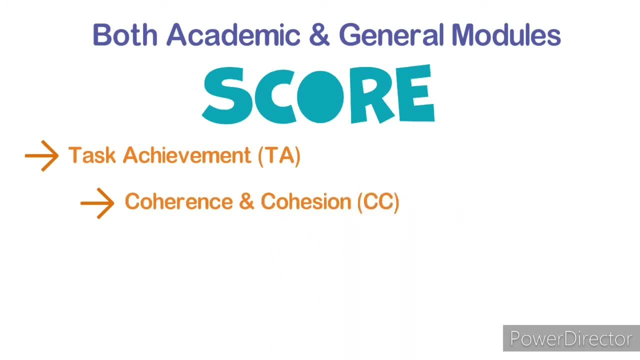 This means you are writing in a good context and your sentence sequence is correct. The third one is lexical resource. This means you have used correct vocabularies and good phrases. The last one is grammar range and accuracy. That means you have used correct grammars in your writing. 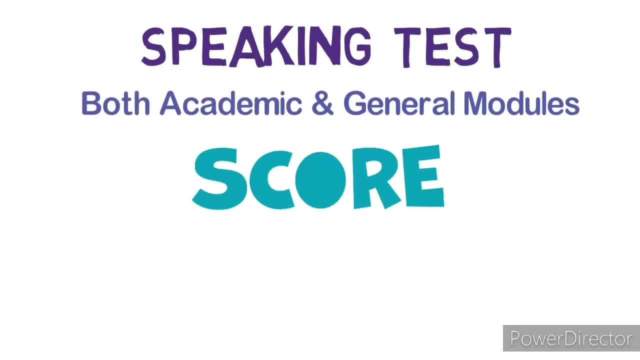 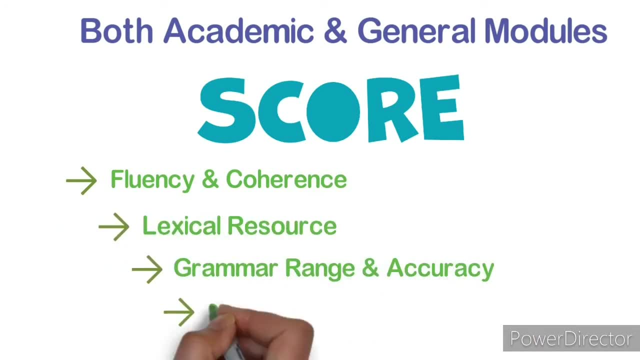 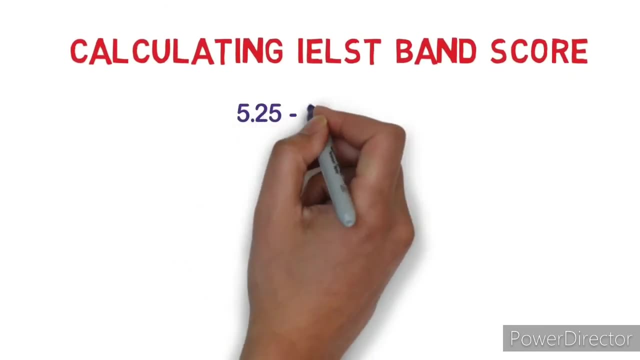 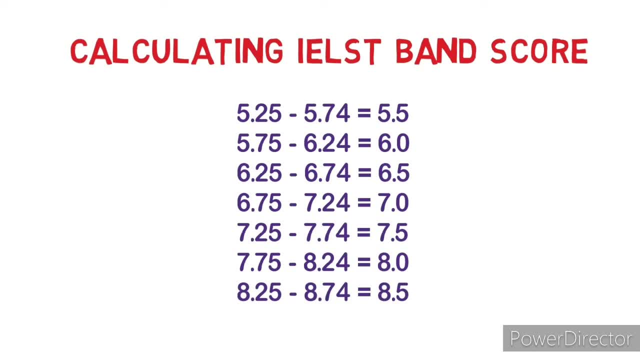 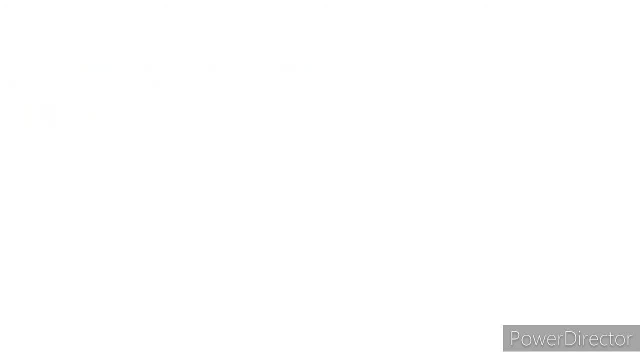 If you get anything between 6.5 and 6.5,, you get 5.5.. If you get anything between 6.75 to 7.24, it is 7.. Your score will be 8.5 if you get anything between 8.25 to 8.74.. 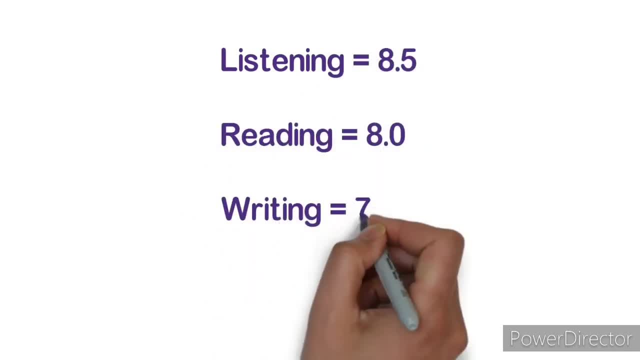 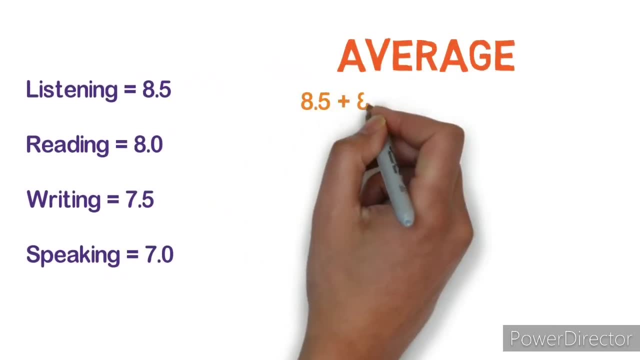 For example, suppose you got 8.5 in the listening test, 8 in the reading, 7.5 in the writing and 7 in the speaking. So first they will average your score by dividing it by 4.. 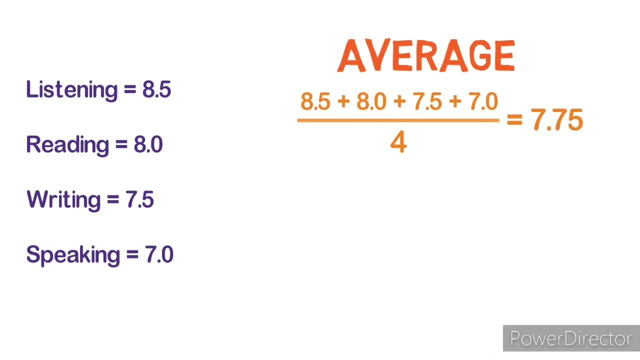 In this case, this will be 7.75.. Now, everything between 7.75 and 7.75 is 7.75. And 8.24 will be 8.. 8.24 will be 8. And 8.24 will be 8.. 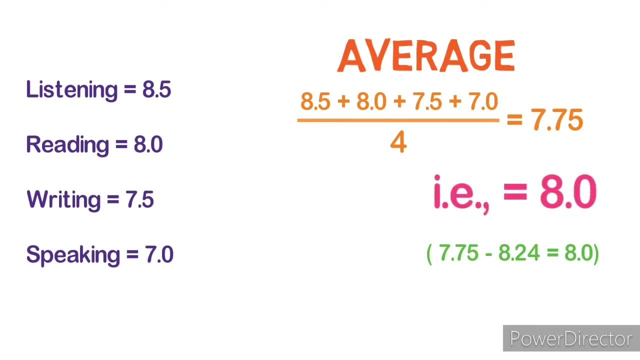 8.24 will be 8. And 8.24 will be 8.. 8.25 will be 8.. 8.25 will be 8.. So your score will be 8.. That means you are a very good user.